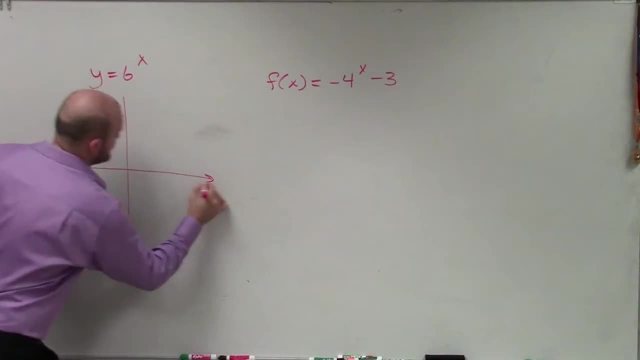 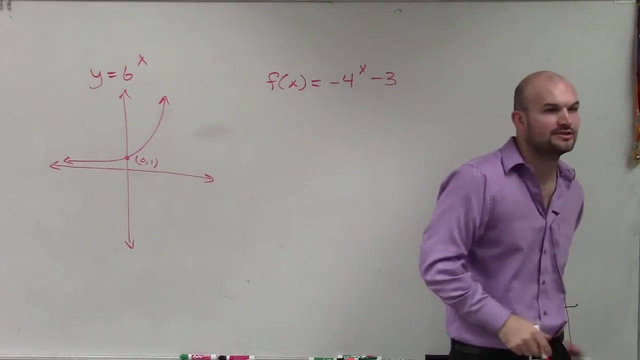 b to the x. When we talked about that, when we looked over exponential functions, this parent graph, remember, has a intercept, a y-intercept at, And the graph looks something like this: Alright, so by looking at this equation, there's a couple things that I want to do. I want 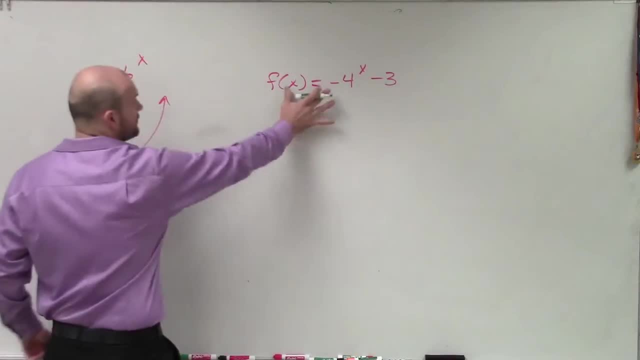 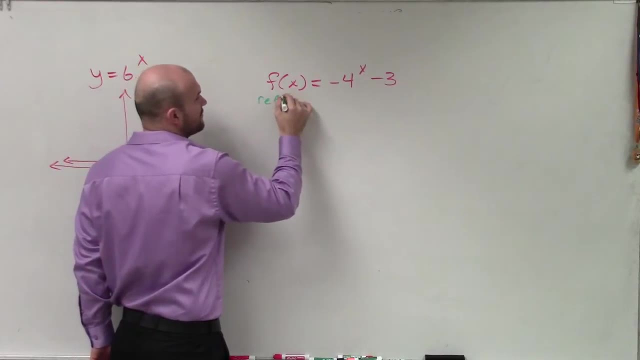 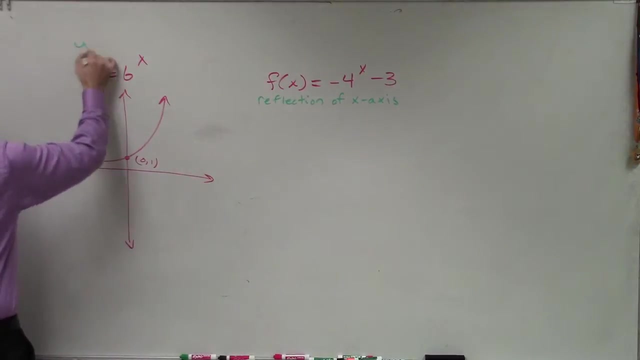 to be able to understand what the transformations are. The first transformation we notice is we have a negative b or a negative a in our standard form. so we know this is going to be a reflection of the x-axis. Right, if we were going to write the standard form, y equals. 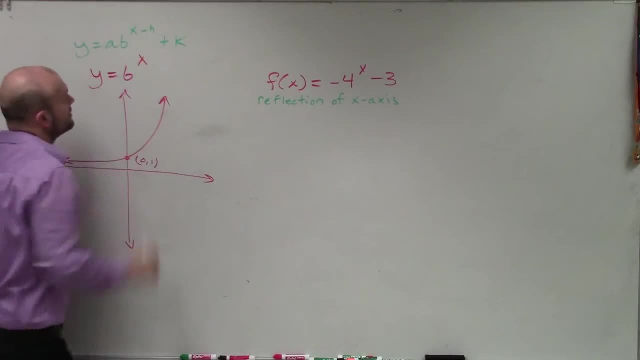 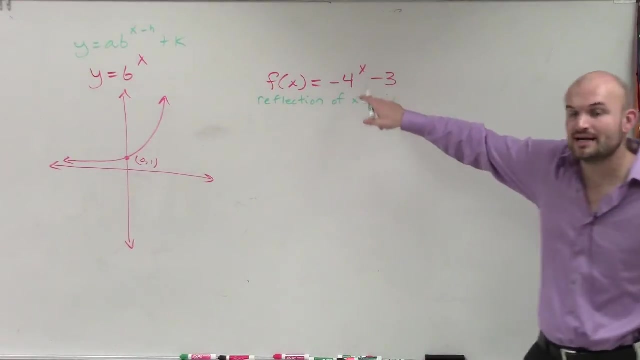 a to the b to the x, minus h plus k. Right, that negative a, just like a quadratic, is going to tell you the graph is going to be reflected over the x-axis. Then this minus three is your minus k, That's. 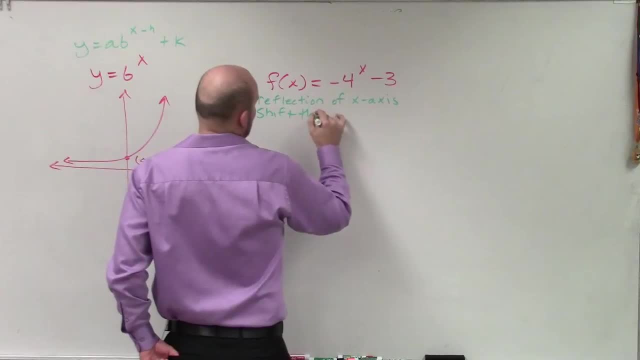 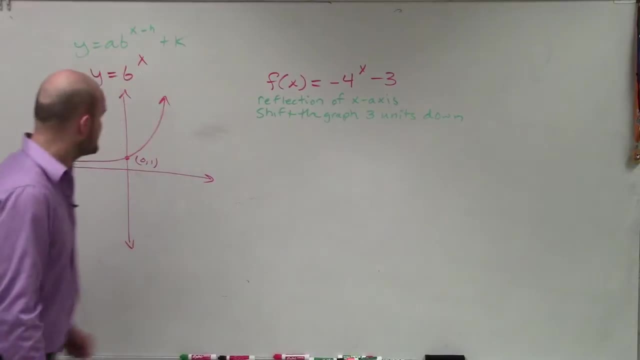 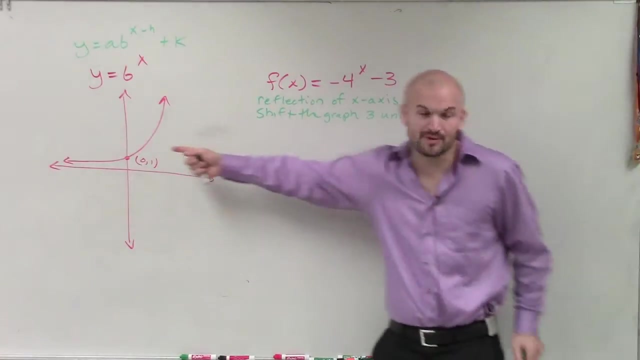 going to tell you to shift the graph three units down. So there's a couple ways you guys can do this. One way is you guys could simply just look into reflecting this parent graph and then shifting it three units down- The other way that I've told you guys to look. 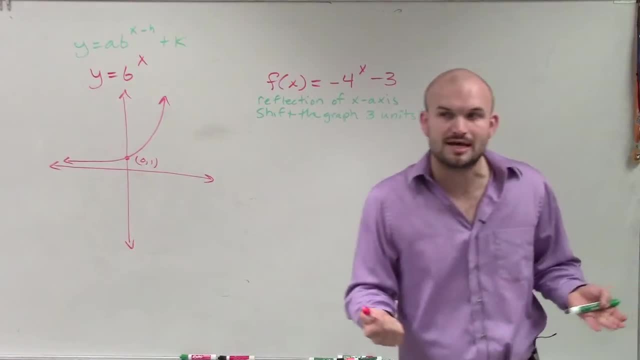 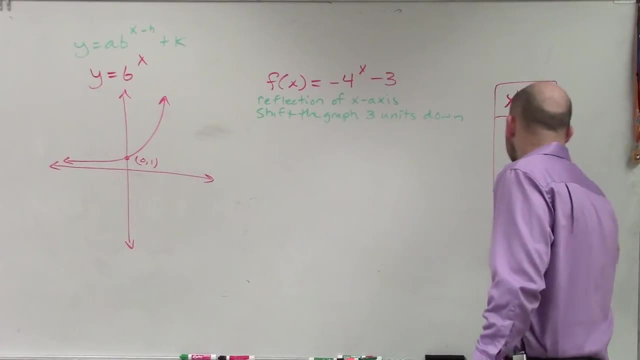 at this is to Just create a table of values, And you don't have to get crazy on your table of values When we're doing a table of values, just pick two points. You don't need anything crazy for your amount of table of values. 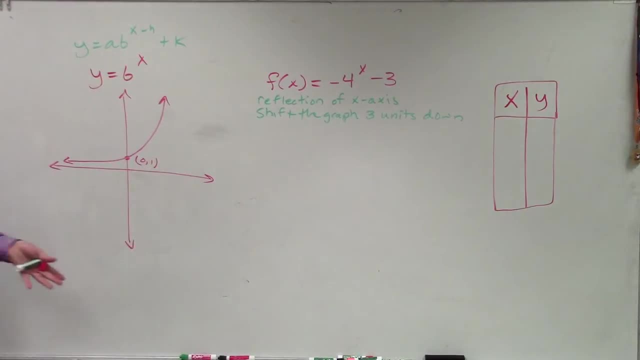 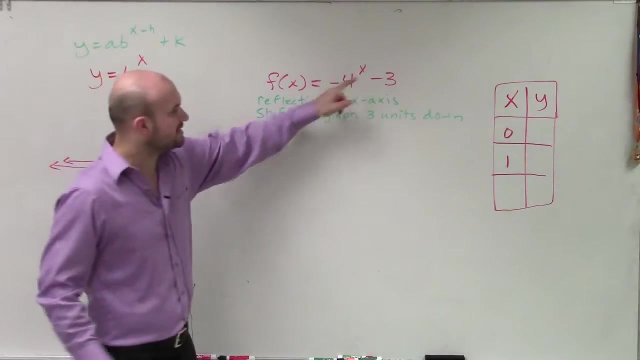 Just pick two points that I'm going to use, And the best two points I told you guys to use is to always go back and use 0 and 1.. Just use 0 and 1.. So when we plug in 0 into this case, what I'll have? 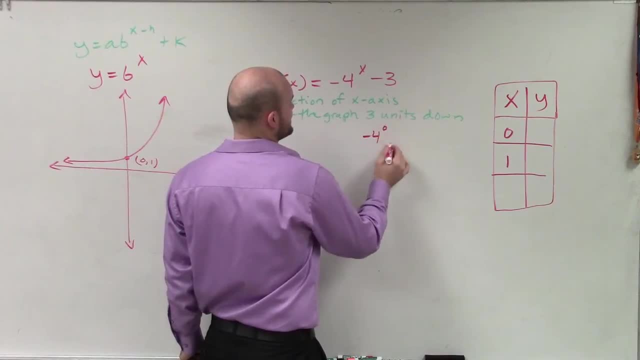 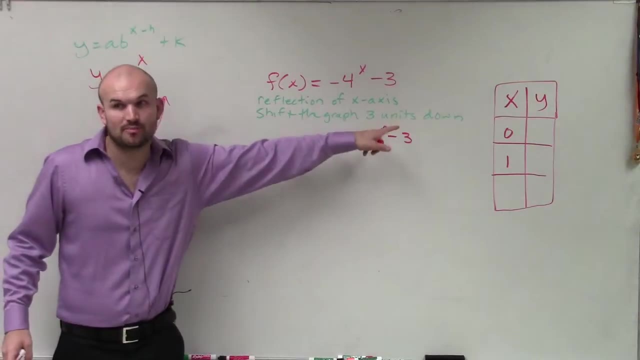 is a negative 4 raised to the 0 power minus 3.. Now remember you're raising 4 to the 0 power, then multiplying it by 0. So 4 to the 0 power is 1.. 1 times negative. 1 is now negative 1.. 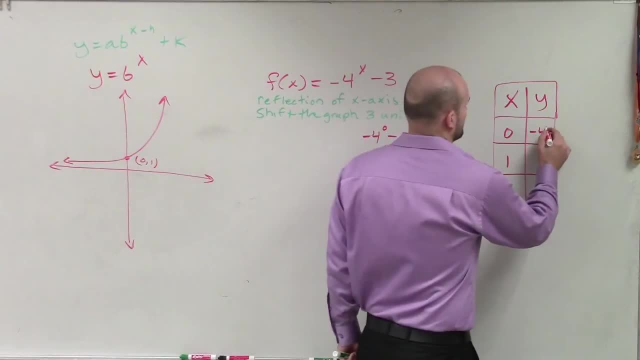 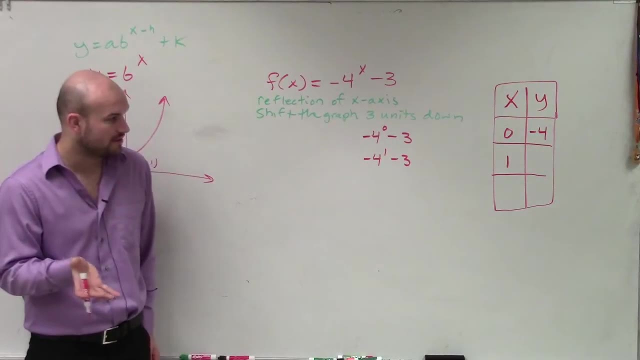 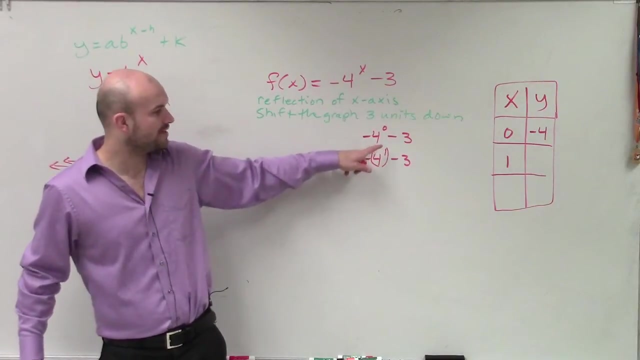 Negative 1 minus 3 is going to be a negative 4.. Then let's do to the first power. Again, It's positive 4.. This, remember, order of operations tells you to do exponents first, then multiplication. So it's 4 raised to the first power, which is just 4,.